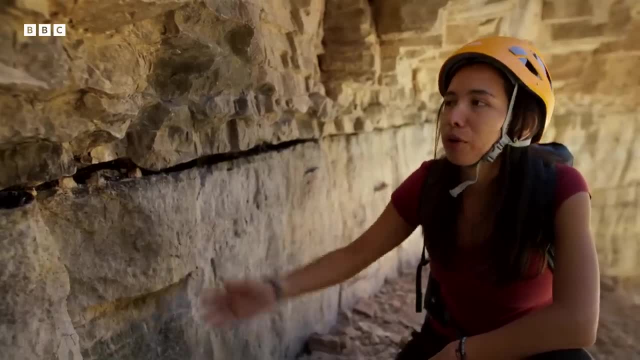 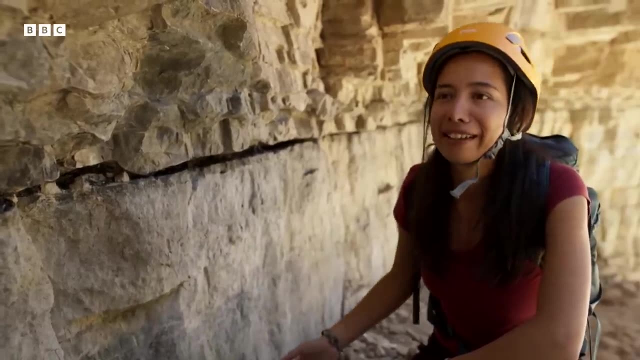 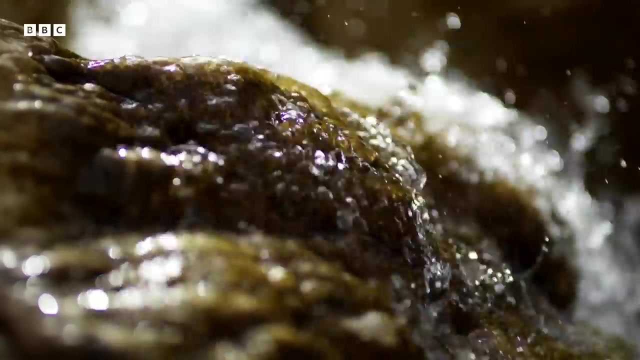 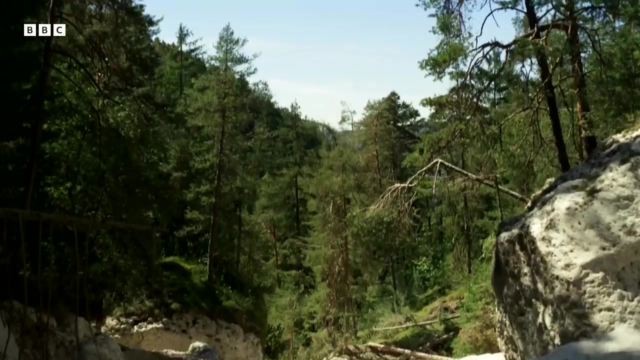 This event- it's not only found here, but also across the planet- Life just vanish. You will see this line of that. You will see how life seems to just vanish. How could volcanic eruptions in the north wipe out so much life across the entire planet? And just see how it's like here. There's a huge history behind this And this is really something that's really really important to us. This really is a really important piece of history. There's an important piece of history that's in the story of the middle of this planet. because the Three-Tailed River, the three-tailed river that we live in, and the three-tailed river has been just around that corner. It's just a piece of history, so we don't have a long way to go about it. Let's just look at it one more time and we're going to talk a little bit more about that, Okay, And then I was wondering- maybe this is your favorite part of that story- Is there a three-tailed river? Yes, Okay, Okay. 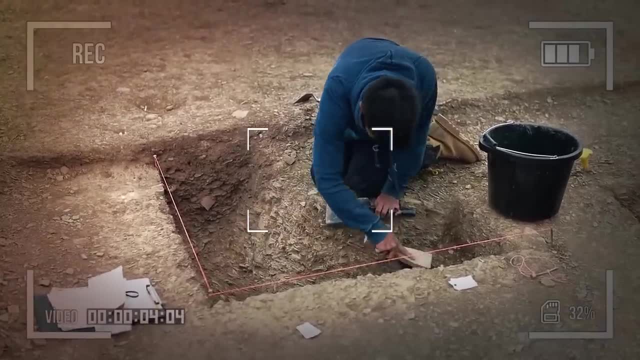 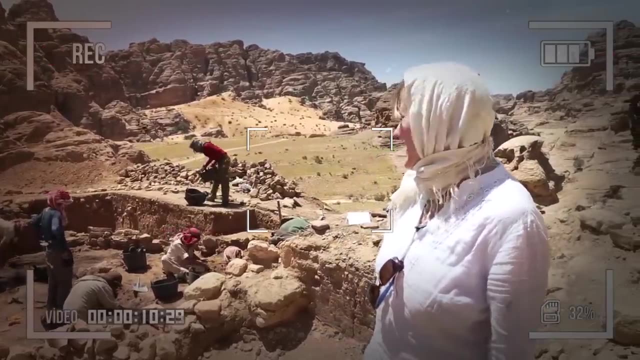 Throughout the ages, archaeologists and historians have dug up remnants of lost civilizations. You never know what you're going to dig up and it's just nice and calm and peaceful, and. but you get those moments where it's very exciting when you find that thing. 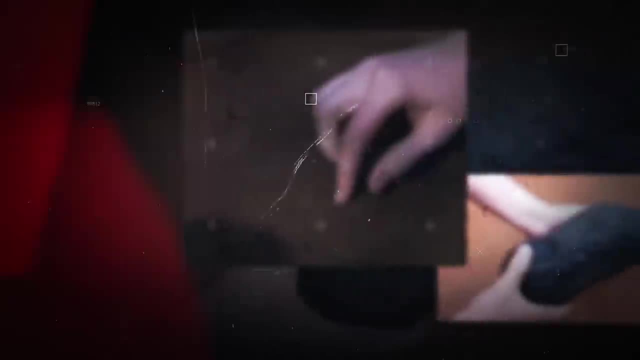 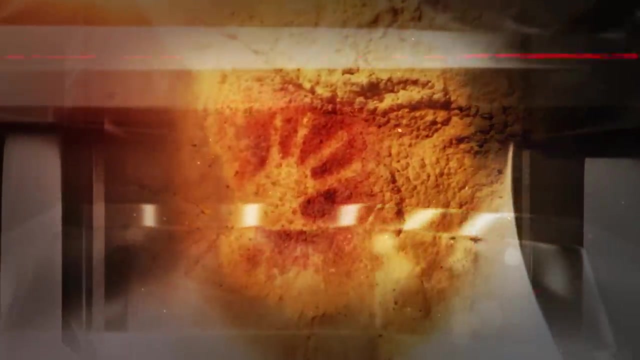 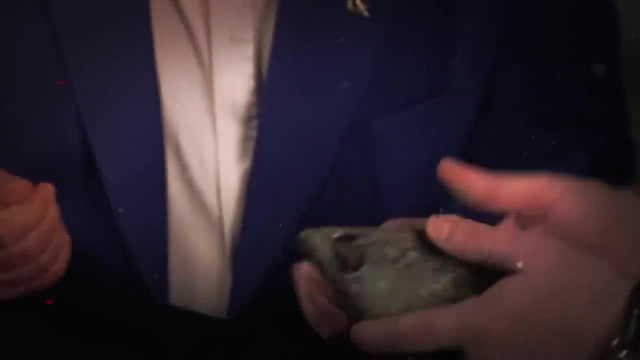 Piecing together the puzzle of humanity's past. Yet amidst the rubble and dust lie artifacts that defy explanation, Discoveries that threaten to rewrite the very fabric of history itself. What are some examples of forbidden archaeological finds throughout history, And who decides which discoveries are off-limits to researchers, and what motivations might they? 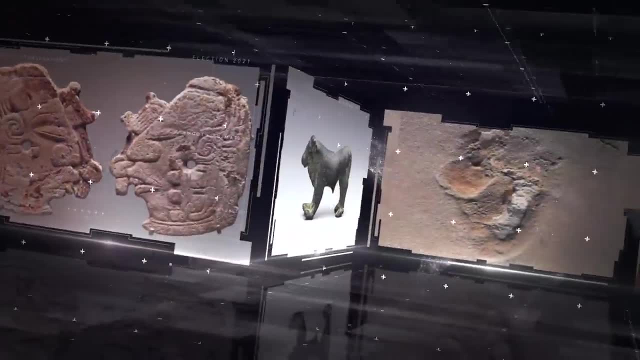 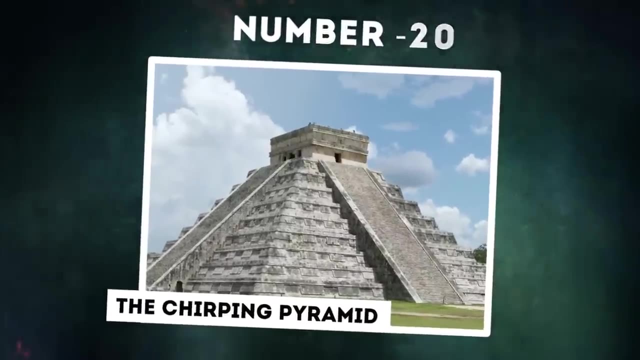 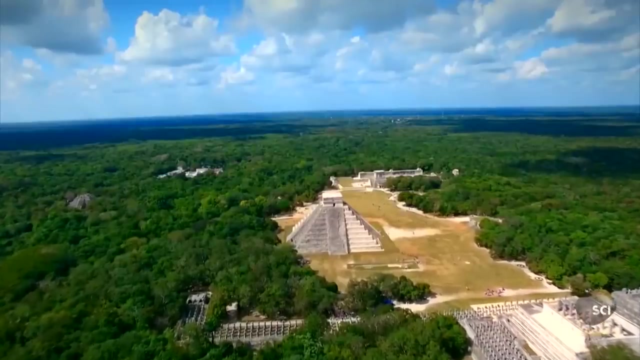 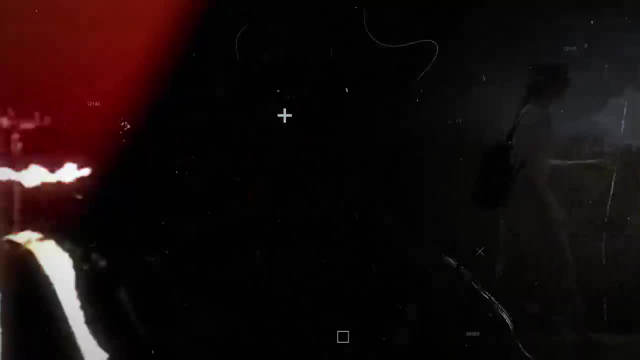 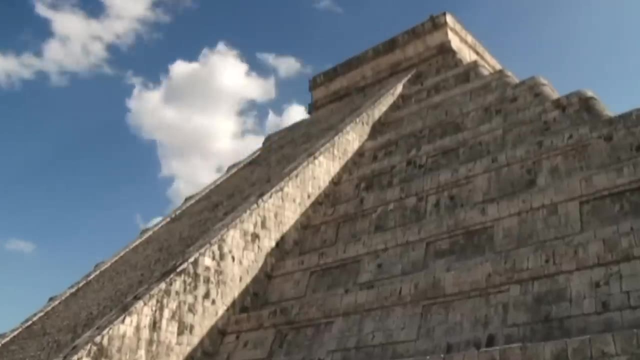 stone. The pyramid is made of stone. The pyramid is made of stone. The pyramid is made of stone. An extraordinary sound reverberates back, A sound reminiscent of the sacred clear birds call deeply revered in Maya culture. What makes this auditory experience even more intriguing? 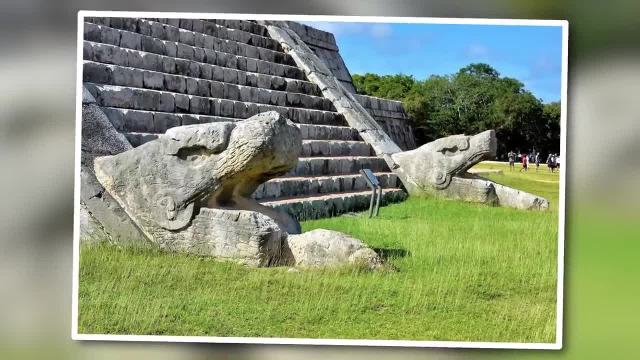 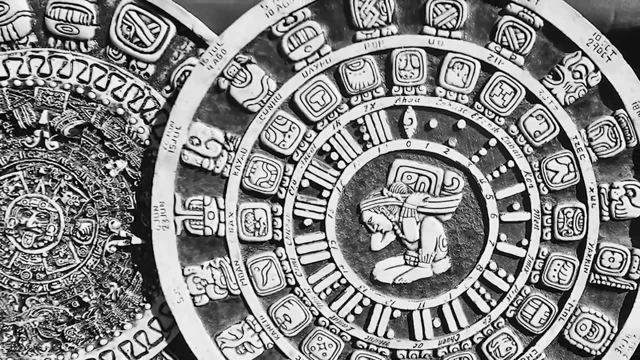 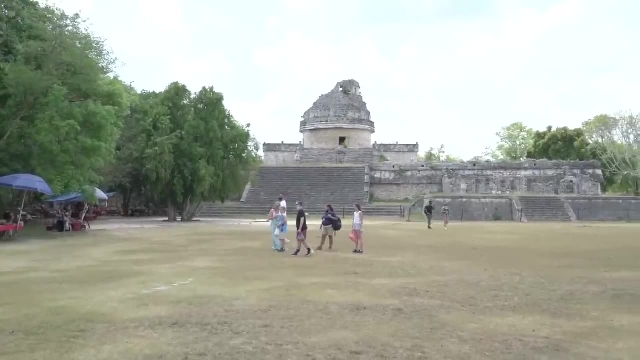 is the pyramid's unique design. It boasts four stairways, each adorned with 91 steps, amounting to a total of 365 steps, A direct reflection of the days in the Maya calendar. This architectural symmetry isn't just for show. It plays a pivotal role in creating the mysterious.